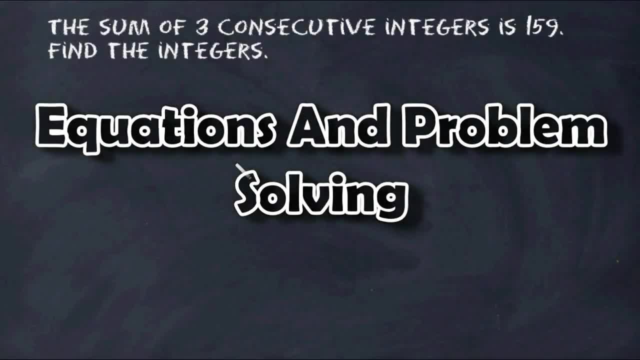 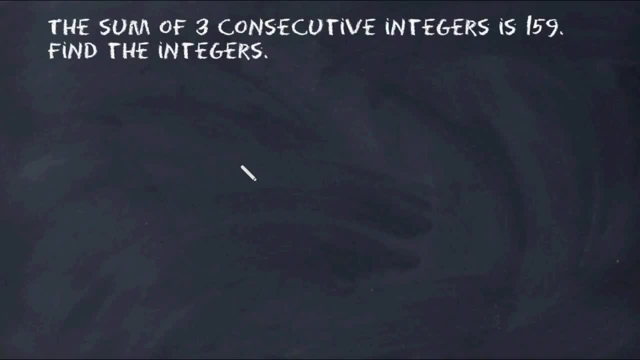 Hello everyone, this is Mr Masonette, and in this tutorial we are going to demonstrate how you can use equations to problem solve. This problem is saying that the sum of three consecutive integers is 159 and we have to figure out what those three consecutive integers 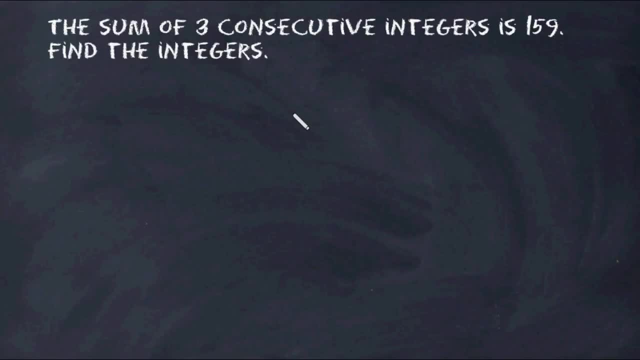 are Now. by consecutive they mean in a row. For example, the numbers 1, 2 and 3 are three consecutive integers, or 9,, 10 and 11 is another example. Now we could just experiment and write three random consecutive integers and see if they total 159, but that might take. 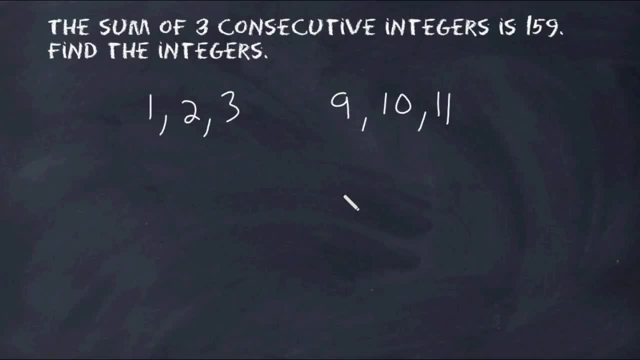 quite a while. So what we're going to do is we are going to write an algebraic equation to represent the situation and then solve. Now it is not given what any of the integers are, So what we're going to do is we are going to use the variable. 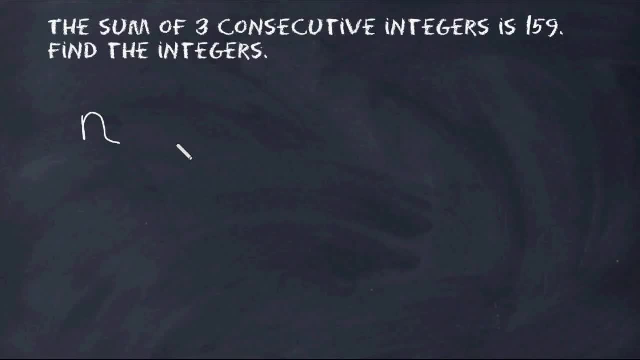 n to represent whatever the first integer is. Now, because we know that the next number would just be the first one increased by one, we can just write that as n increased by one or n plus 1.. And we know that the third number is going to be two larger than the first one. 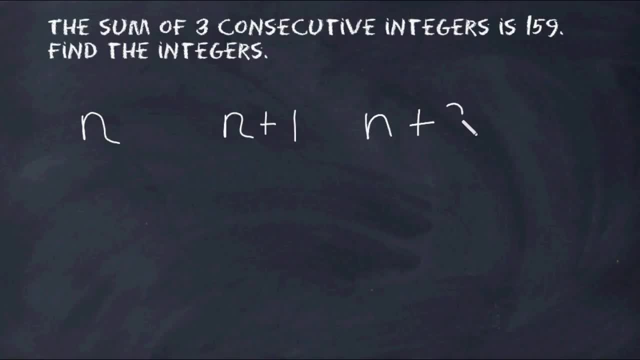 so we're going to write n plus 2.. And just to kind of show the nature of this, let's just write three consecutive integers like 5, 6 and 7, and let us look at the number 6 and understand that it really is just 5 increased by 1, and 7 really is just 5 increased by 2.. So whatever. 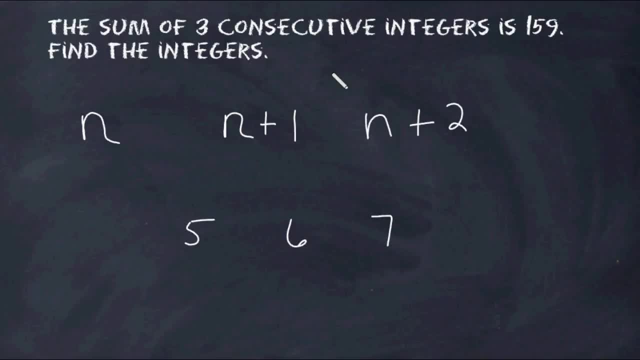 the second number is: is the first one increased by 1, and whatever the third number is is just the first number increased by 2.. So now we have to take whatever our first integer is and add it to the second integer and add that to the 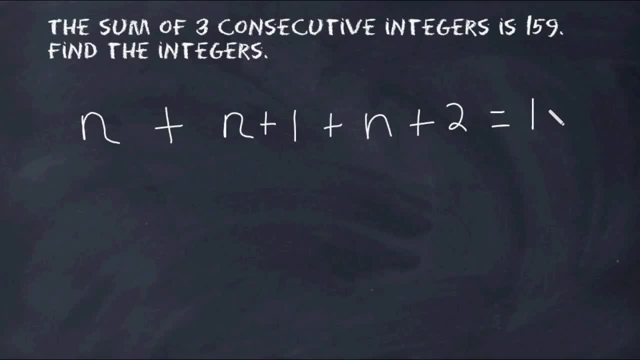 third integer and that will have a sum of 159.. Now we have an equation where we can solve for n and figure out what the first integer actually is. Next we have to combine like terms. we have one, two, three n's in our equation, so we